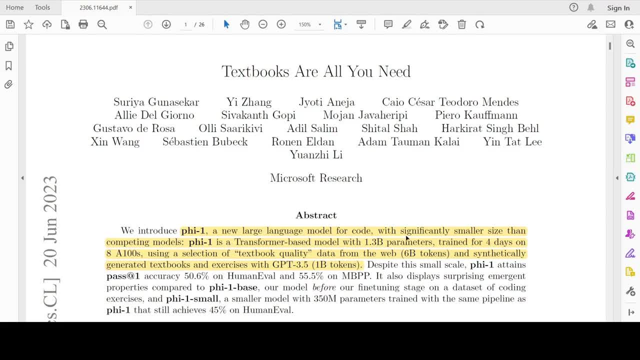 It is a transformer based model with just 1.3 billion parameters. And it has been trained for 4 days on 8 A100s using a selection of textbook quality data from the web, 6 billion tokens and synthetically generated textbooks and exercises with GPT 3.5, 1 billion tokens, so totally 7 billion tokens of training data. 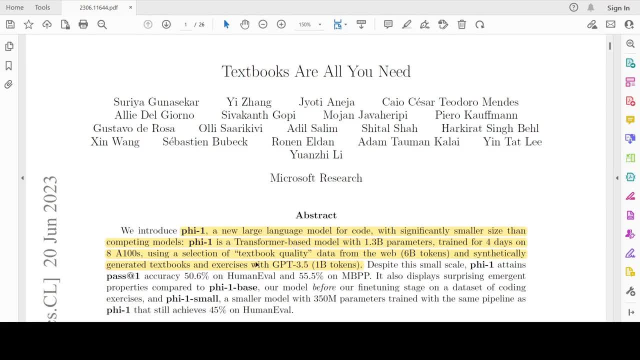 Okay, so what is special about this 1.3 billion parameter model? Okay, so what they say over here is that when compared to models of much higher sizes, okay, like say, your codex 12 billion, which is 12 billion parameters or wizard coder 16 billion parameters, right? This gives comparatively very good performance. Wizard coder 16 billion parameters on a data set size of 1 trillion tokens on this human eval password accuracy. It gives comparatively very good performance. 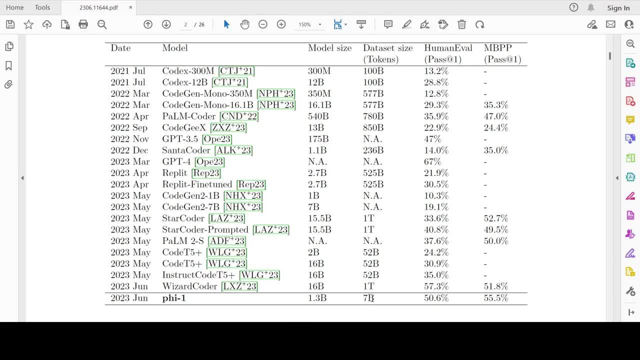 It gives 57.3 whereas Pi 1 with a 7 billion tokens for training and a model size of 1.3 billion parameters is giving 50.6 percentage. Okay. And on this other benchmark MBPP, it is in fact better than wizard coder over here. Okay, so this smaller model is achieving performance comparable to models of much more higher scale. Right? So how did they achieve this? 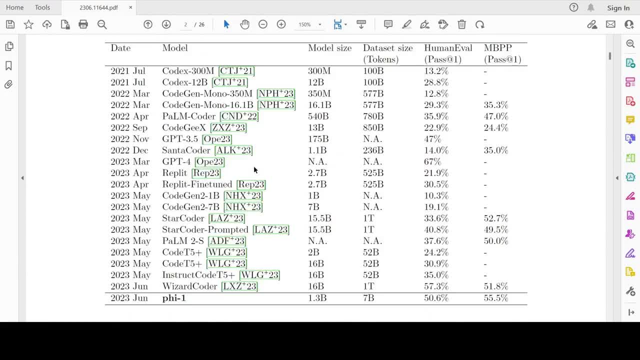 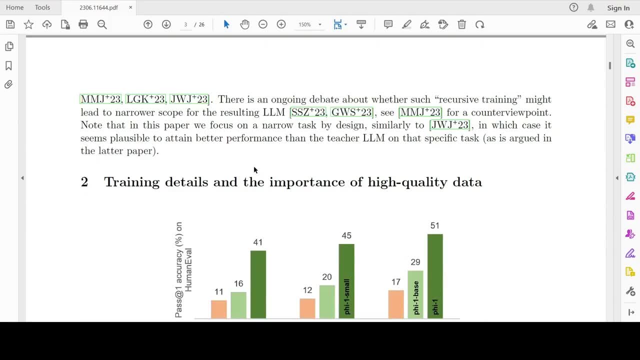 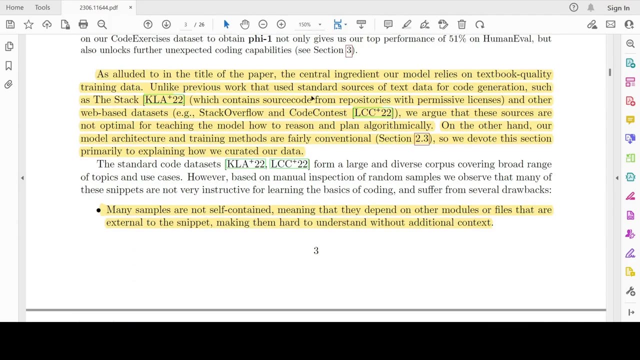 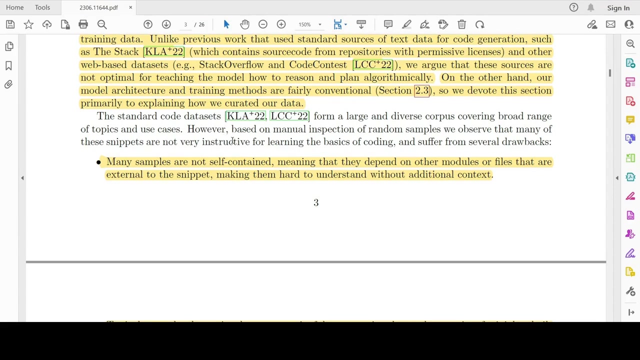 okay so what they are saying over here is that they could achieve this because they used high quality data for training okay so what they are saying over here is that you have these general data for say code generation right standard sources for code are text data for code generation such as the stack okay which contains source codes from repository with permissive licenses and other web-based data sets like stack overflow and code contest these sources are not optimal for teaching the model how to reason and plan algorithmically okay so what they are saying is that current corpuses which are available right they cover a large broad range of topics and use cases but based on manual inspiration 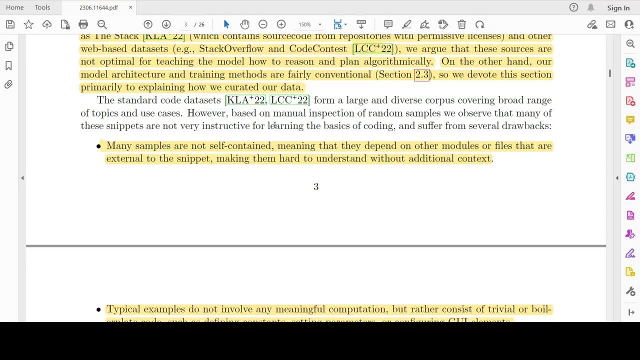 what they are saying is there are several drawbacks for you know learning the basics of coding this suffers there are these snippets code snippets have some drawbacks like many samples 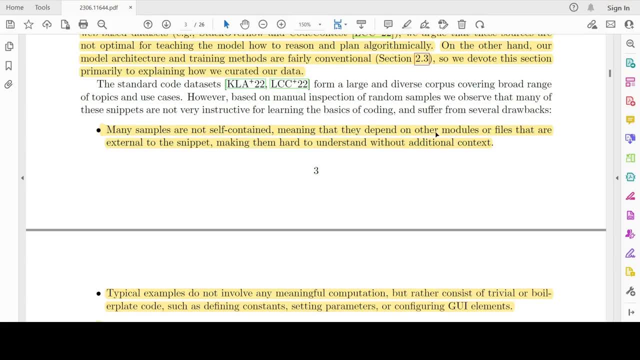 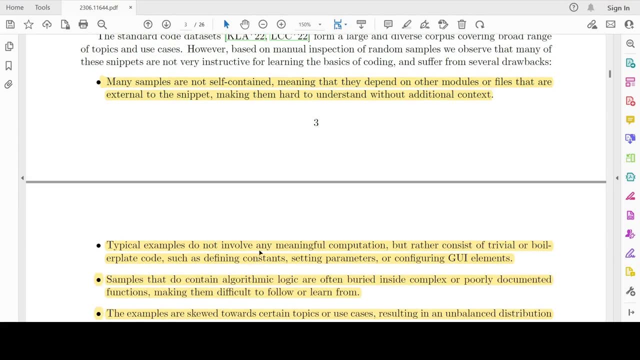 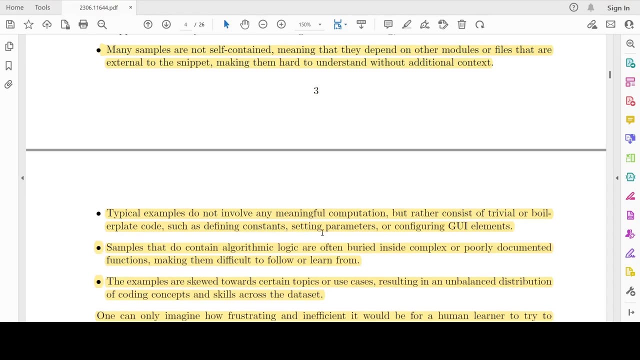 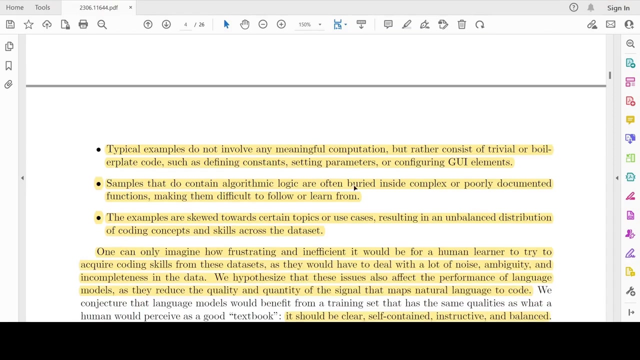 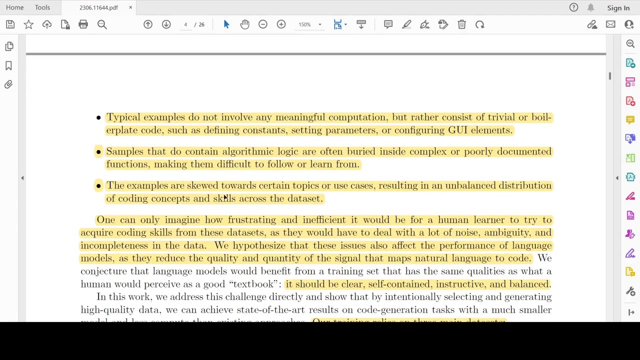 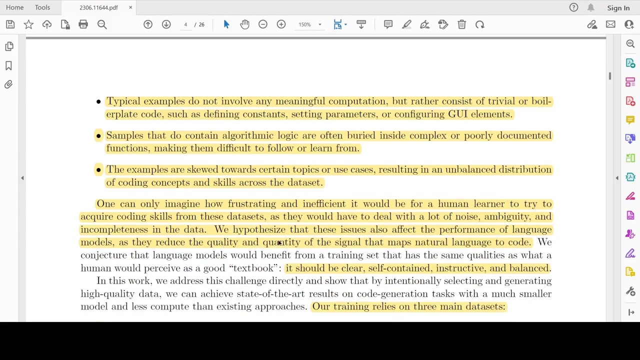 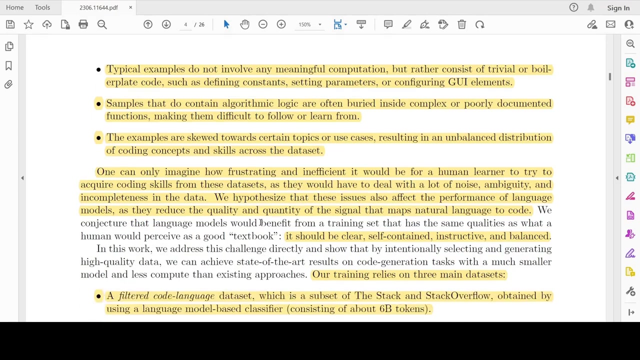 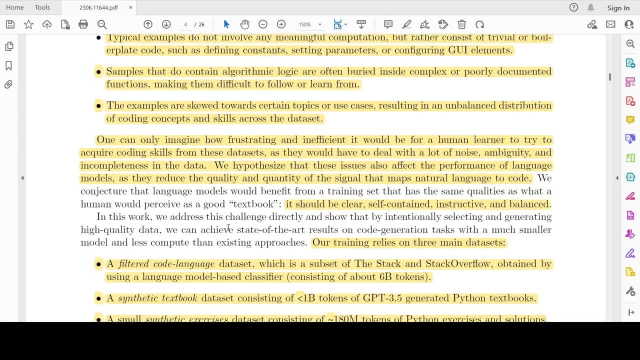 instructive and balanced okay so they address this challenge directly and show that by intentionally selecting and generating high quality data we can achieve state-of-art results on code 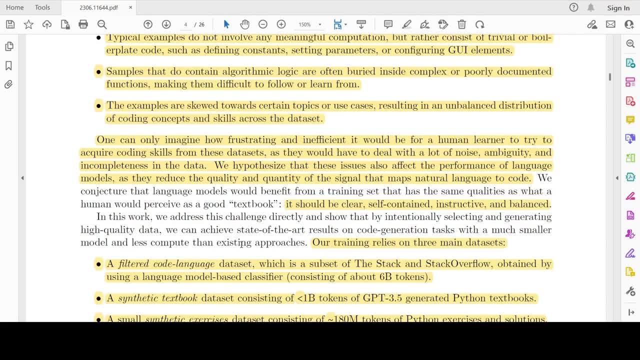 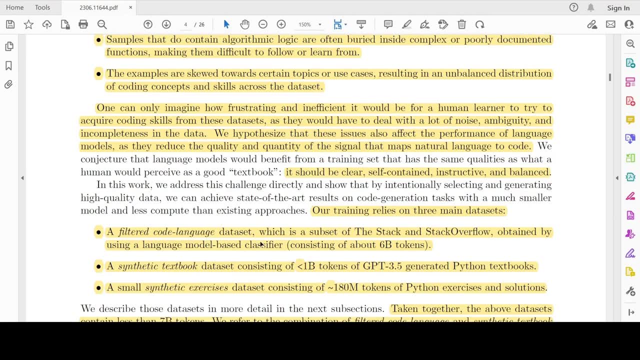 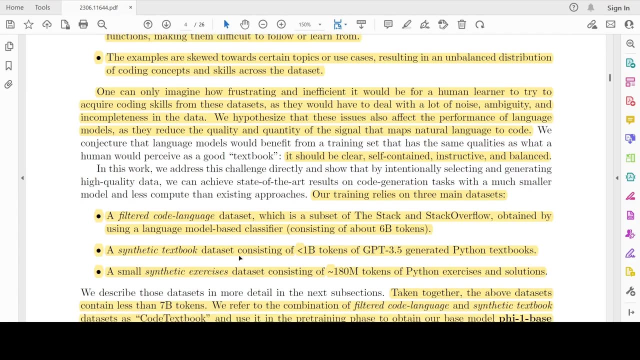 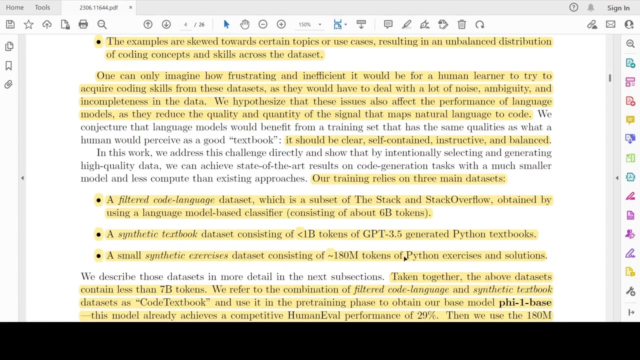 generation tasks with a much smaller model and less compute than existing approaches so they rely on three main data sets a filtered code language data set which is a subset of the stack and stack overflow obtained by using a language model classifier about six billion tokens a synthetic textbook data set consisting of less than one billion tokens of gpt 3.5 generated python textbook a small synthetic exercise data set consisting of 180 million tokens of python exercise and solutions okay taken together this comes close to 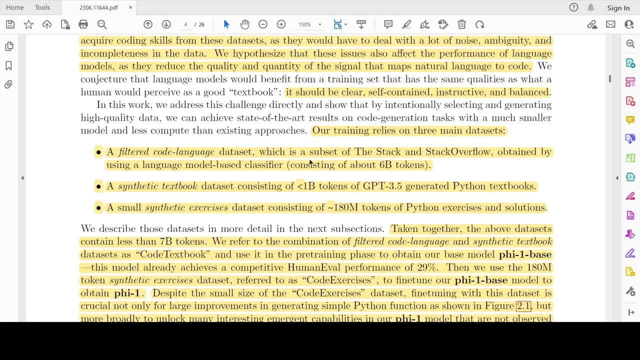 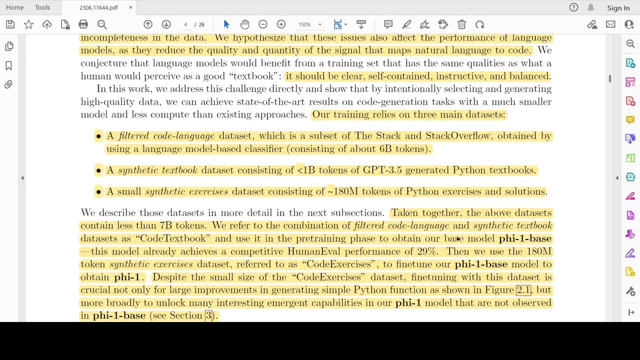 seven billion tokens of gpt 3.5 generated python textbook a small synthetic exercise 7 billion tokens so they refer to the combination of filtered code language and synthetic textbook as code textbook and use it in the pre-training phase to obtain phi 1 base okay it achieves already a competitive human eval performance of 29 then they use the remaining 180 million tokens to fine-tune it and that they call as phi 1 okay and this is showing much better performance of say 50 percent on human eval okay 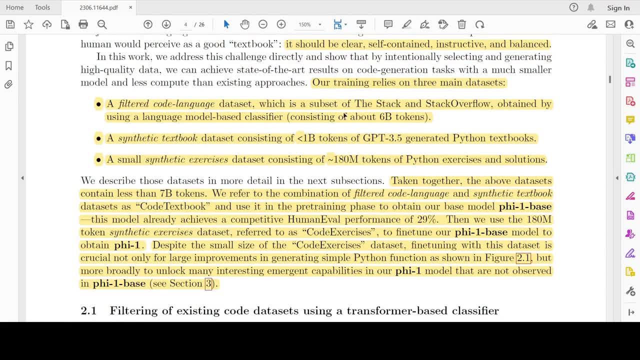 so that is the key thing over here how this data set was created and what is this textbook 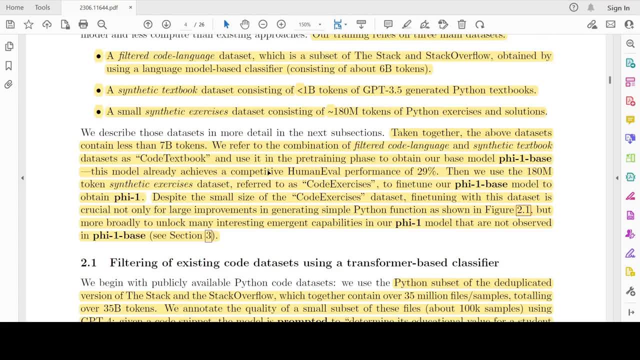 quality data set okay that is one huge insight from this particular paper and the insight that if you have good quality data, even smaller models can give you comparable performance 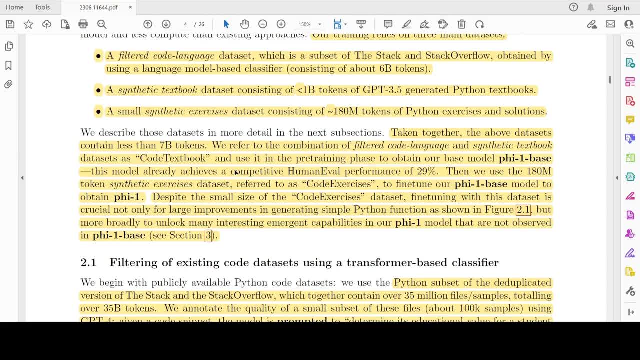 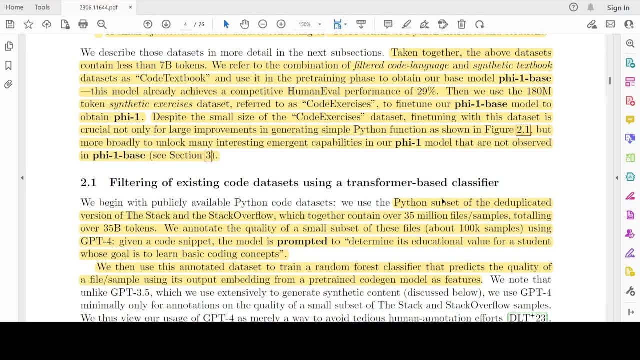 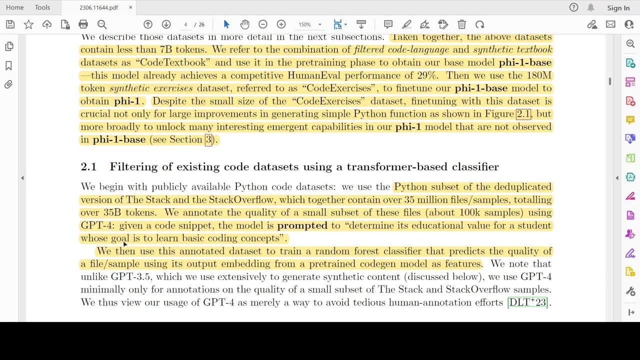 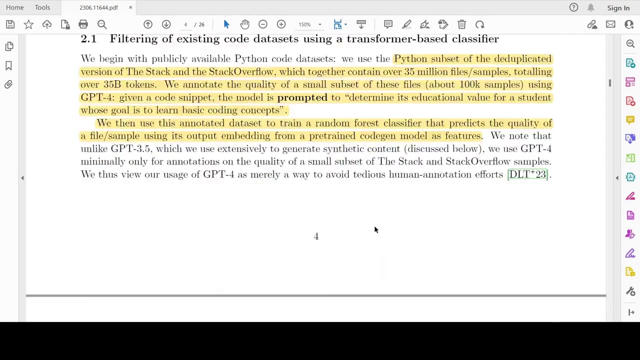 to larger models okay so for our filtering of existing code data set. What they use this transformer based classifier. rhythms programs code. so they took data from the stack and stackoverflow some 100k samples and they used gpt4 to classify you know to get a quality of the code whether to determine whether it is educational value for a student whose goal is to learn basic coding concepts so here is an example so given 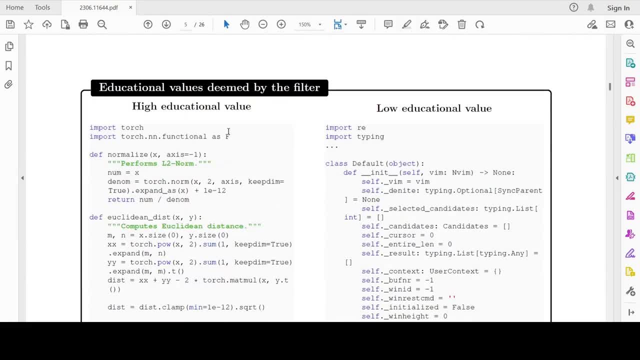 this kind of a code these two code gpt4 will classify some of the code as high educational value and some of the things low educational value it will not classify but it will tell 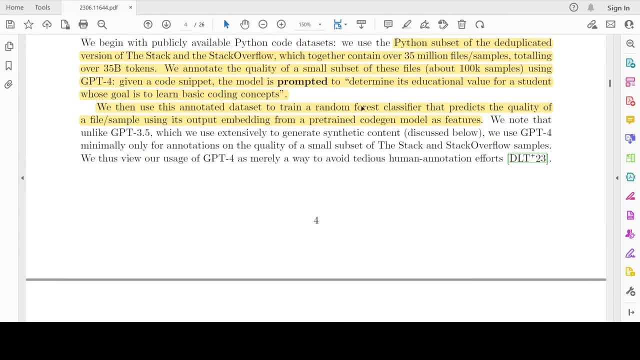 right then what they did was on that annotated data set they trained a random forest classifier that predicts the quality of a file sample using its output embedding from a pre-trained 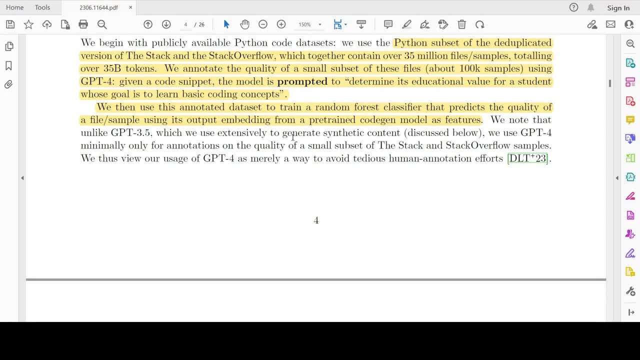 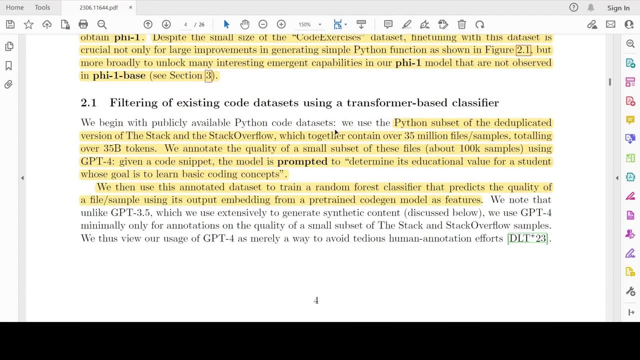 code gen model as features so then they used this to actually collect data of high quality okay they use this classifier to collect data of high quality from the stack and the stackoverflow okay so this is close to 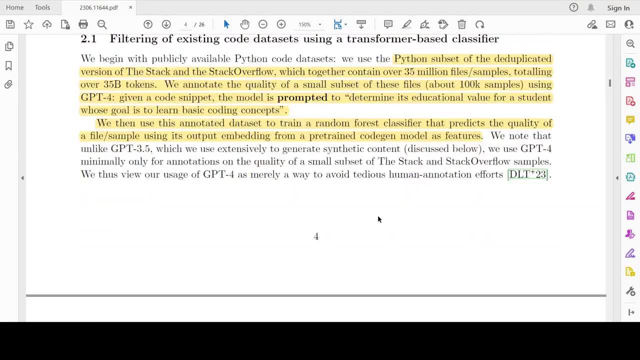 signal billion tokens right so that is what is explained over here the next is creation 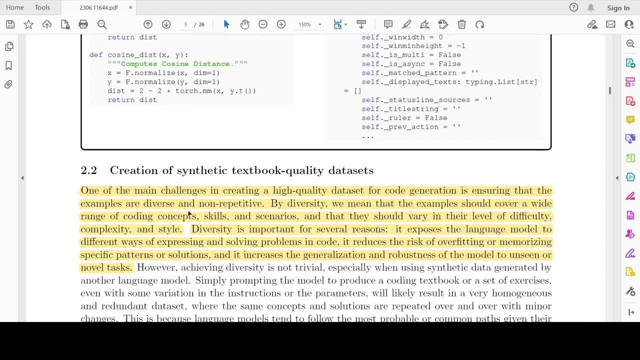 of synthetic textbook quality data set okay so one of the main challenges in creating high quality data set for code generation is example should be diverse and non repetitive okay so basically the examples should vary in their level of 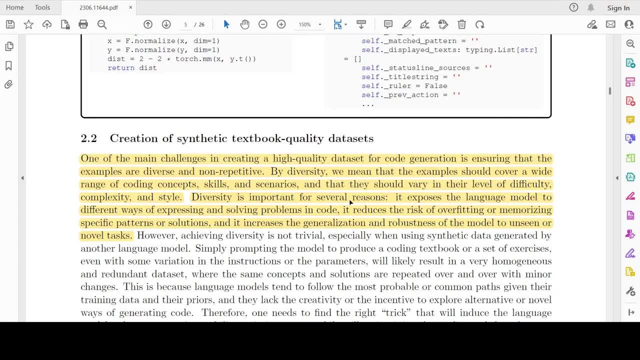 difficulty complexity and style so diverse one only when your data set is diverse then the language model can learn different ways of expressing and 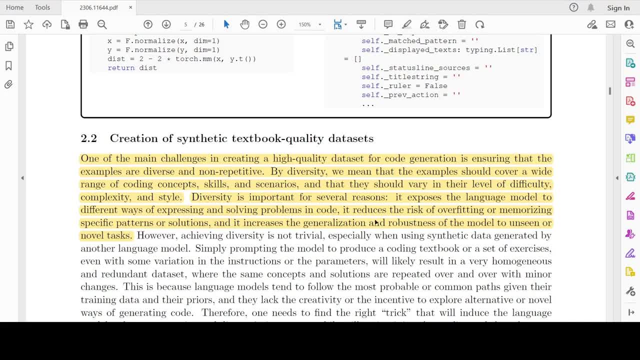 solving problems in code it reduces the risk of overfitting or memorizing specific patterns or solutions and increases the generalization and 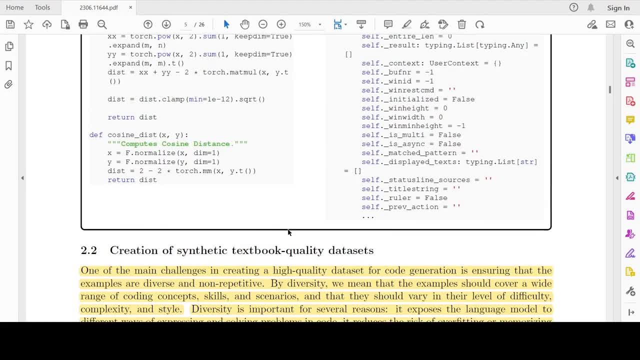 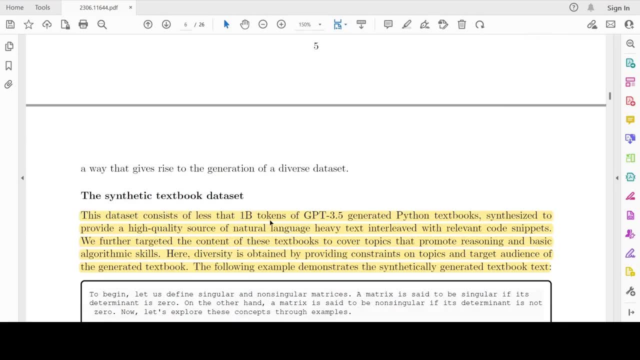 robustness of the model to unseen or novel tasks okay so here they have this data set consists of 1 billion tokens of GPT 3.5 generated Python textbooks 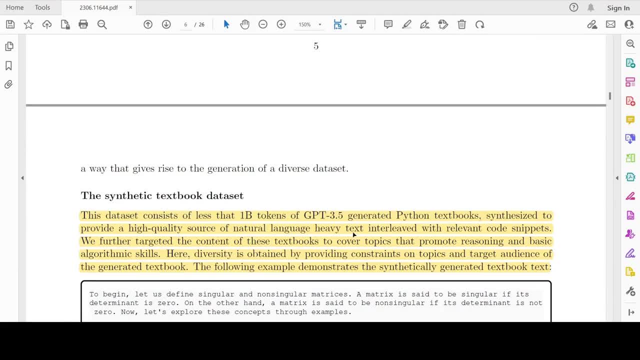 synthesized to produce high quality source of natural language heavy text interleaved with relevant code snippets 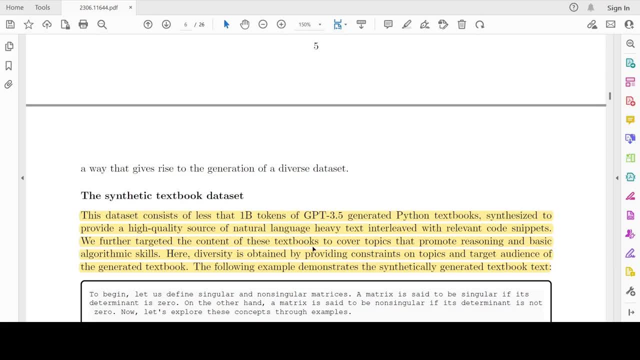 we further target the content of these textbooks to cover topics that promote reasoning and basic algorithm skills diversity is obtained by providing constraints on topics and target audience of the generated textbook so 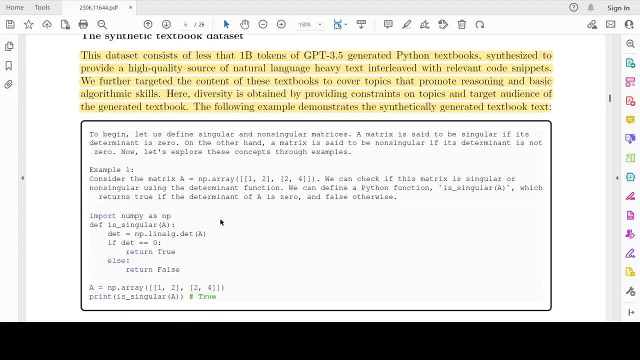 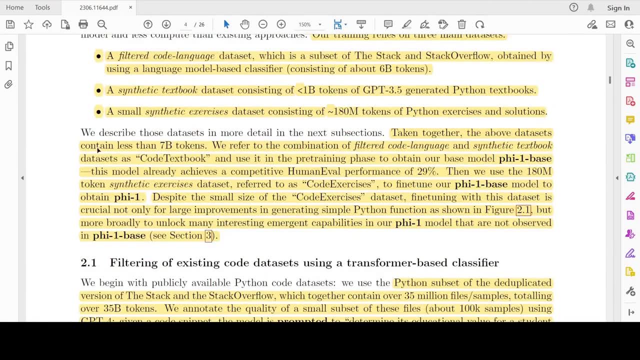 here is an example of a synthetic generated textbook text okay they use GPT 3.5 for this so this is another 1 billion tokens of text okay 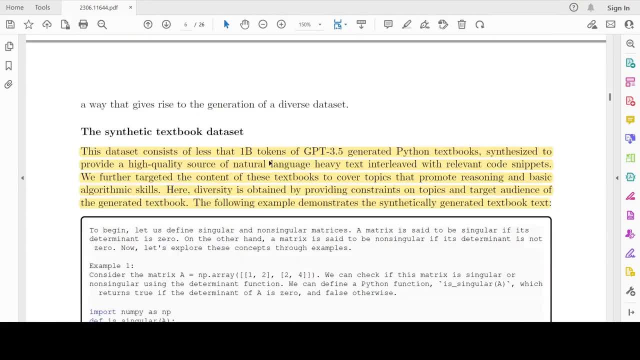 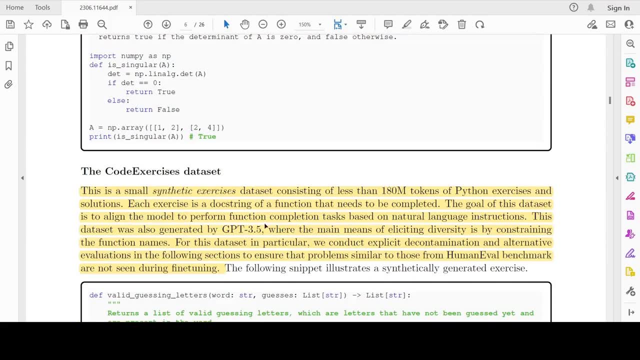 then they also generated synthetic exercises okay the code exercise data set okay the goal of this data set is to align the model to perform function 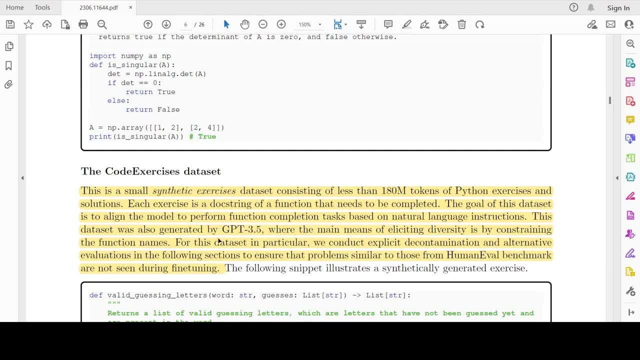 complete tasks based on natural language instruction this data set was also generated by GPT 3.5 where the main means of eliciting diversity is by 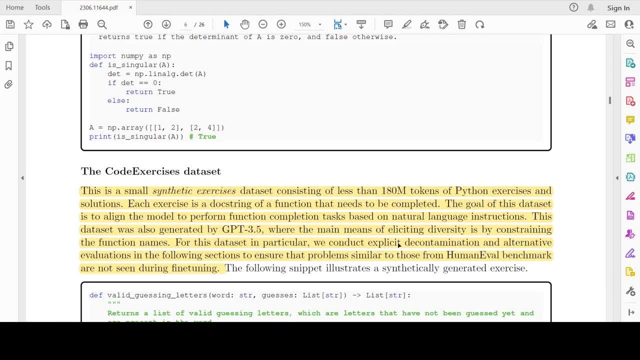 constraining the function names okay they conducted explicit decontamination and alternate evaluations in the following to ensure that these problems 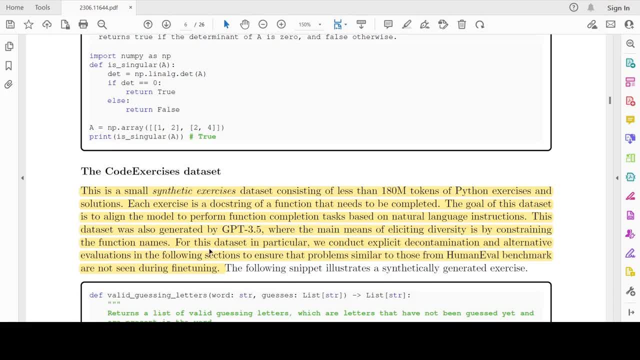 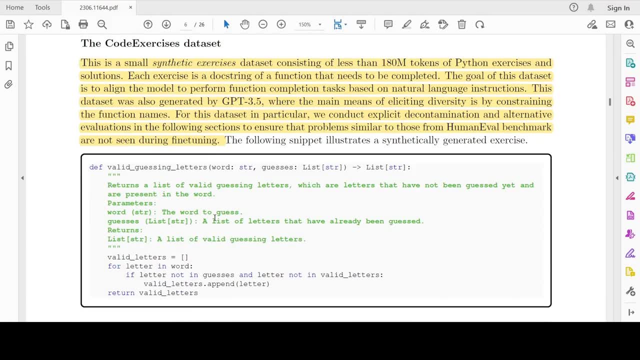 similar to human evolve of network are not seen during fine tuning okay so this is a example after synthetically generated exercise 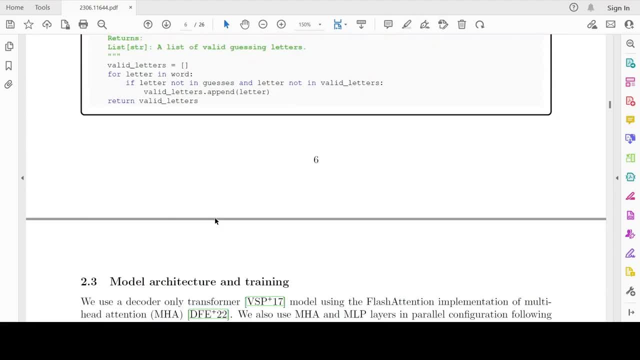 they created this code exercise data set for fine tuning so this was about data so the model architecture is actually a transformer based architecture 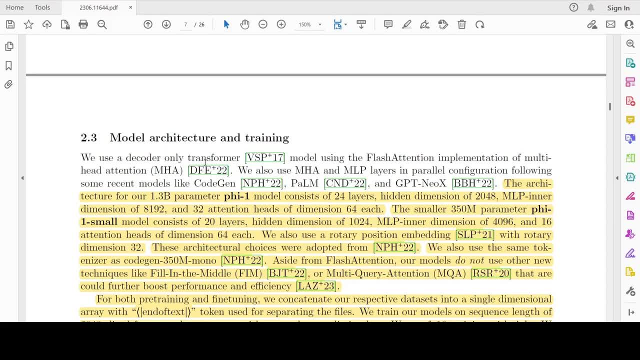 okay decoder only transformer basically VSP plus 17 model using Flash Attention so the architecture consists of 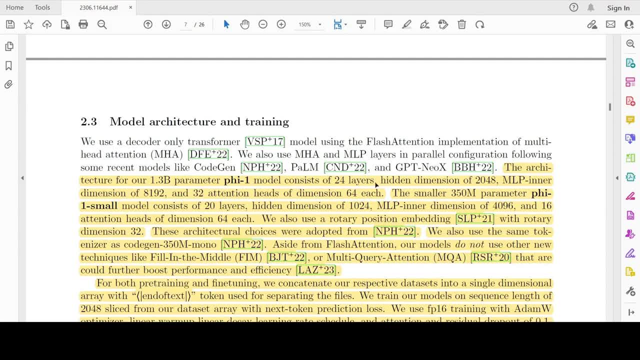 of the 1.3 billion parameter phi 1 module consists of 24 layers hidden dimensions of 2048 mlp inner dimension of 8192 and 32 attention heads of dimension 64 each the smaller 350 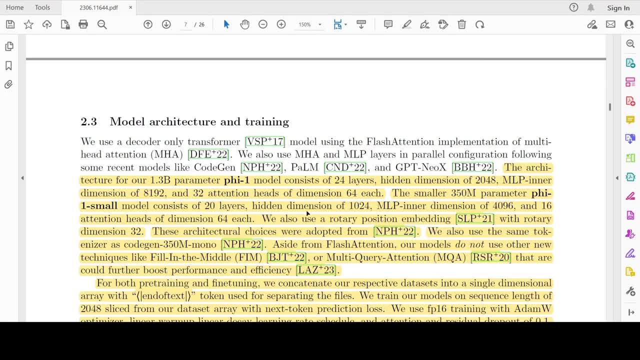 million parameter pi 1 small consists of 20 layers of hidden dimension of 1024 inner dimension of 4096 and 16 attention layers of 64 this thing so they use rotary position embedding 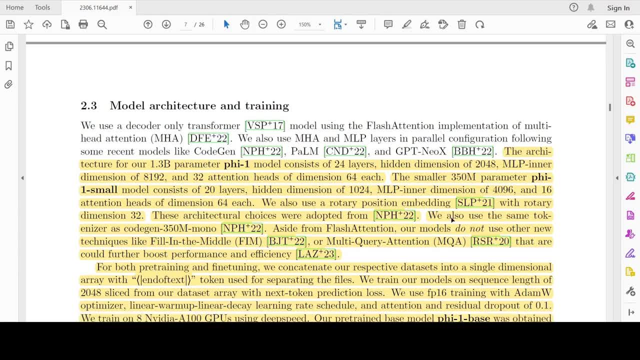 with rotary dimension 32 they use same tokenizer they have adapted from another paper over 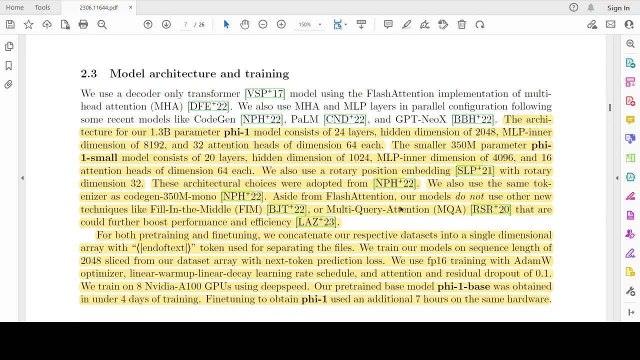 here ok what they say is that apart from do not use the newer fill in the middle or something that could further boost performance and efficiency ok so for both pre-training and fine tuning 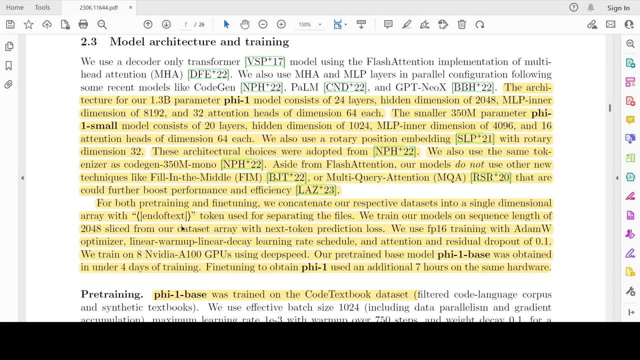 they concatenate respective data sets into a single dimensional array with end of text token used for separating the files ok basically next predi.. 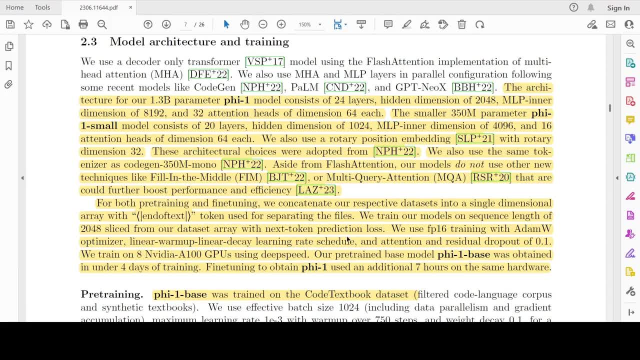 Token prediction. loss is what they are using for pre-training ok once pre-training is done pre-training 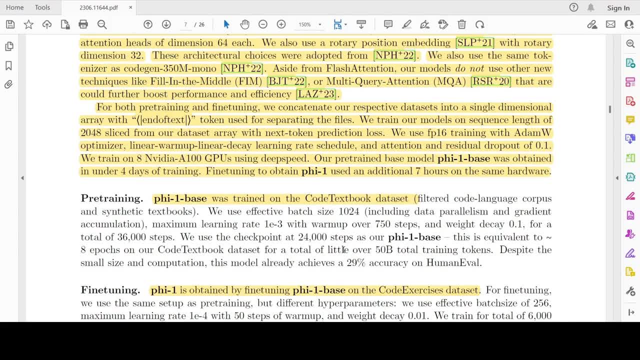 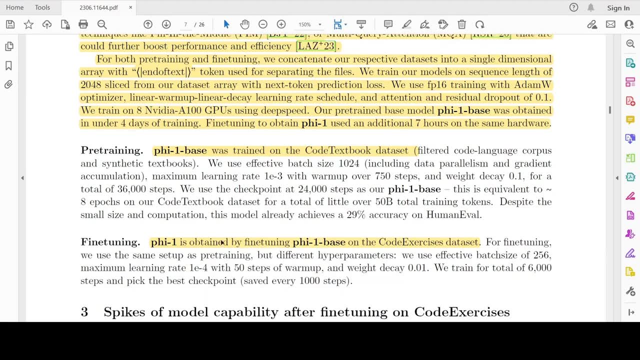 was done on the code textbook data set ok and fine tuning was to obtain phi 1 base right and then they used phi 1 base to actually basically phi 1 is obtained by fine tuning phi 1 base on the code exercises data set that's the idea over here ok then if you see what they are saying is that this phi 1 which has been obtained. 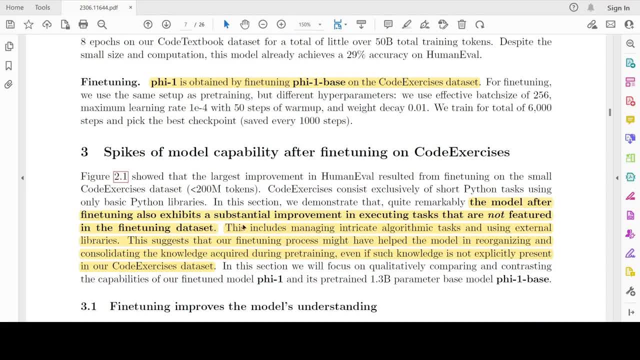 From fine tuning the model also exhibits a substantial improvement in executing tasks that are not featured in the fine tuning data set ok this includes managing intricate algorithm task and using external libraries this suggests that the fine tuning process might have helped the model in reorganizing and consolidating the knowledge acquired during pre-training even if such knowledge is not explicitly present in the code exercises data set. So this is what we have seen in the pre-training data set. So this is what we have seen in the pre-training even if such knowledge is not explicitly present in the code exercises data set. Ok. 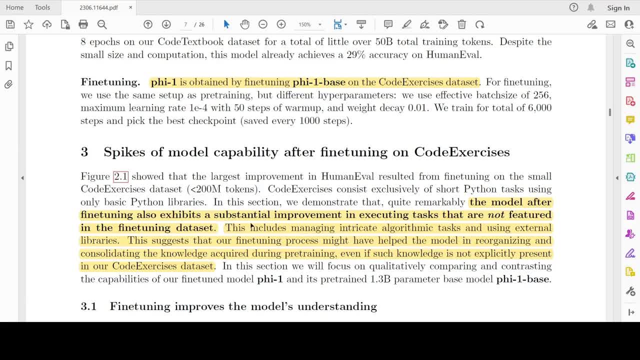 That is one key insight over here that fine tuning improves even out of what you call unseen data basically unseen data tasks which are not seen in the fine tuning data set even that it improves basically. 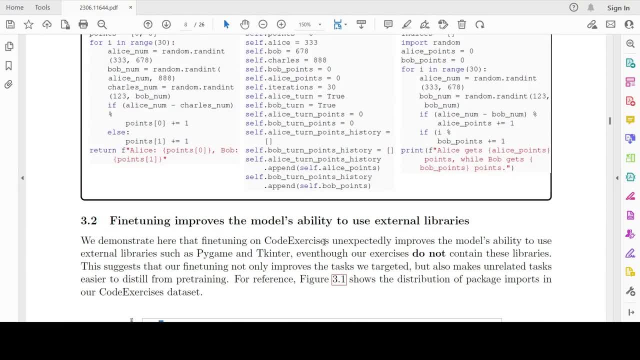 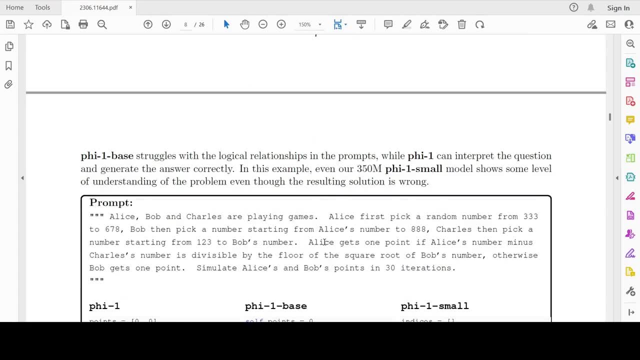 So this is what they talk about over here and then they talk about fine tuning improves the use of model's ability to external libraries, improves the model's understanding. 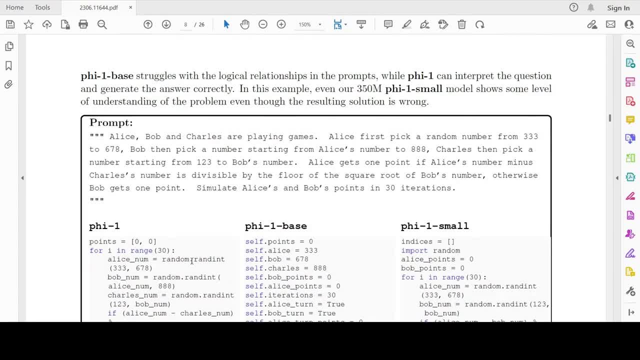 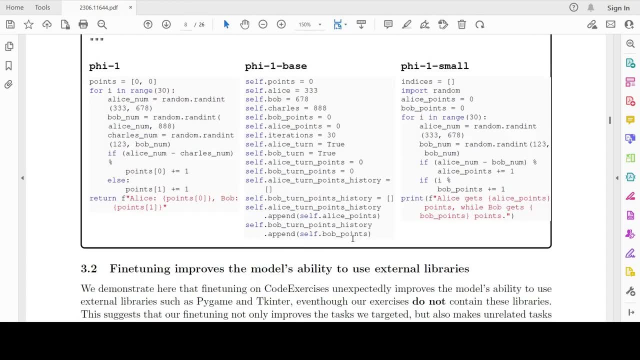 And then they talk about, given a particular prompt, how phi1 improves over phi1 base and phi1 small. That's what they are saying over here. 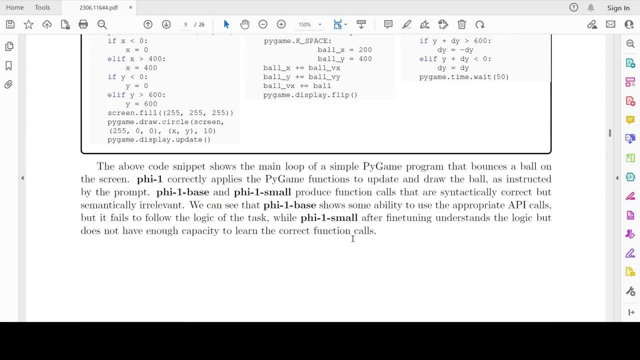 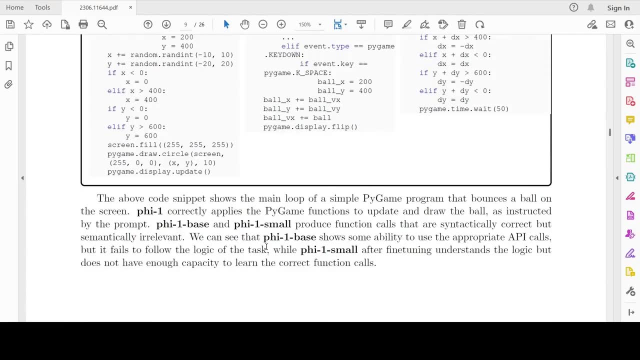 Another interesting thing was this, I'll come to that, where they talk about, a particular use of external libraries over here, like say, write a pi game, there is a ball, this is the prompt. 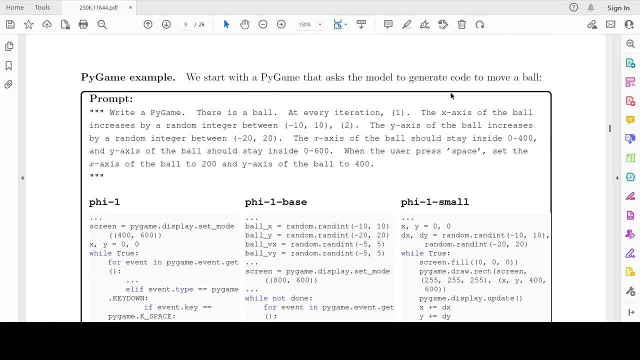 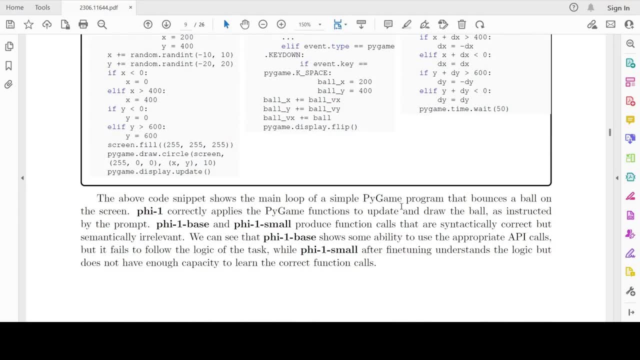 Now, say we start with the pi game that asks the model to generate code to move a ball, so basically that's the prompt, so shows that the main loop of a simple pi game program that bounces a ball on the screen, that is this code snippet, and phi1 correctly applies 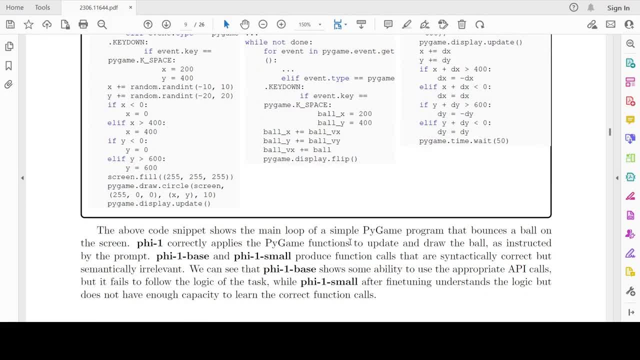 the pi game functions to update and draw the ball as instructed by the prompt. 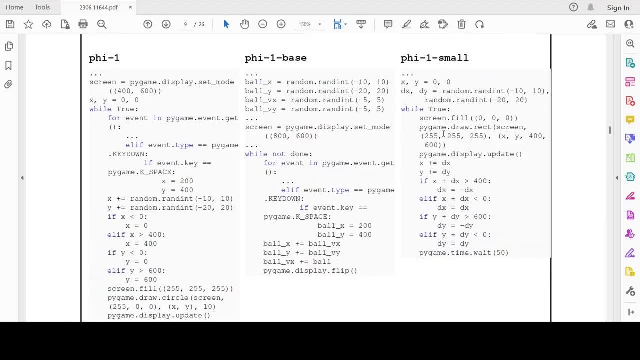 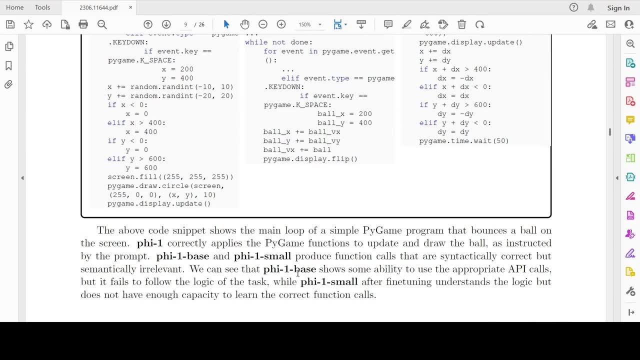 So, phi1 base and phi1 small also produce pi game functions, but they don't work properly. They're syntactically correct, but semantically not irrelevant. 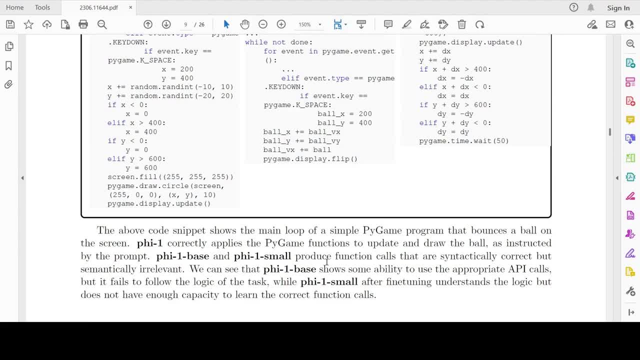 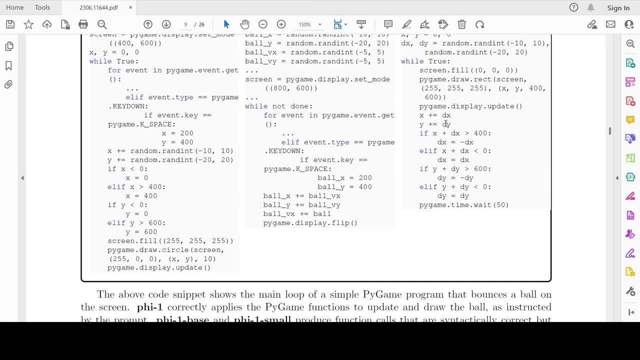 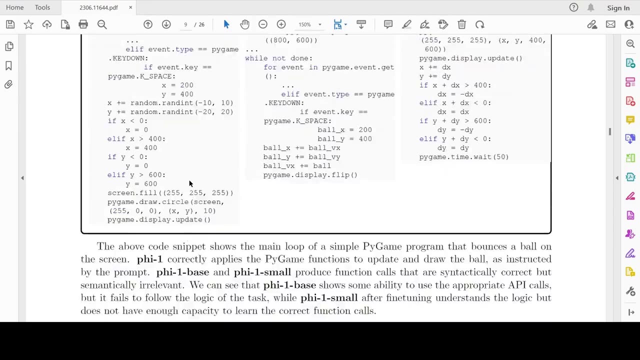 So phi1 is basically, because it is fine-tuned, phi1 small after fine-tuning understands the logic but does not have enough capacity for the correct function calls, whereas phi1 small basically, phi1 gives you better results. So, that's what they are saying over here. 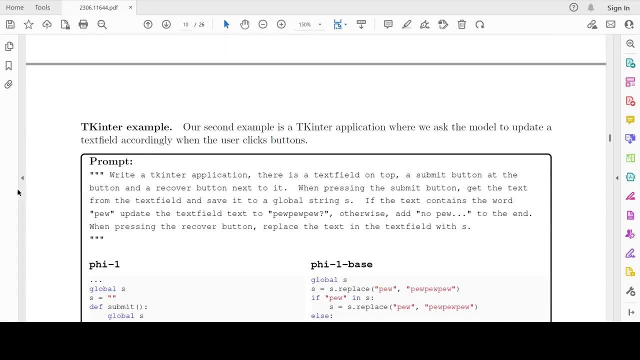 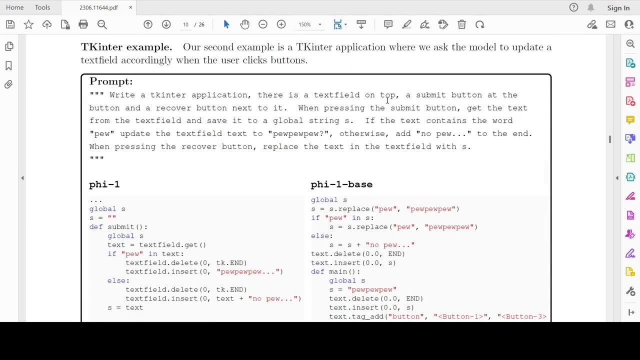 Another example of another tkinter library, again what they say over here is this, write a tkinter application, this is the prompt, there is a text field on top, a submit button at the bottom, I think should be, and a recover button next to it. 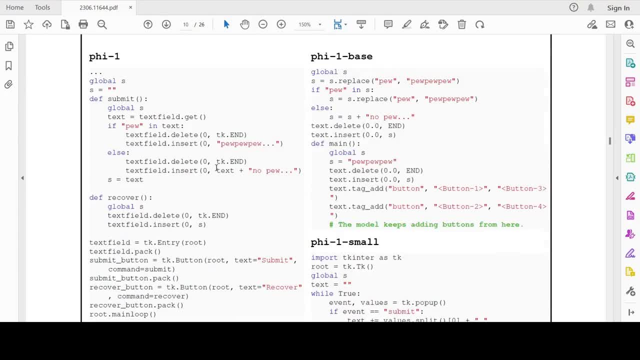 So when pressing the submit button, get the text, so this is what needs to be developed. Here also they say that phi1, both phi1 base and phi1 small failed to use the correct tinker APIs, but phi1 implements the correct functions properly. So, this is what they say over here. 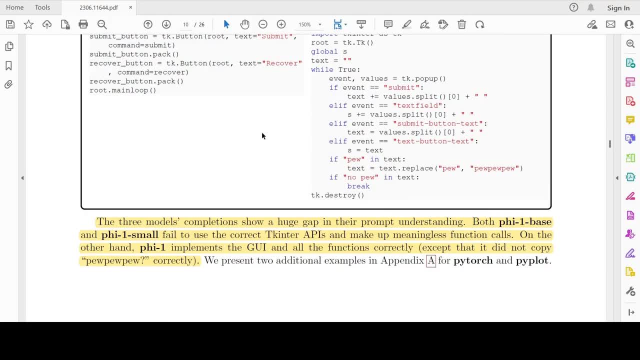 They have some additional examples of pytorch and pyplot also. 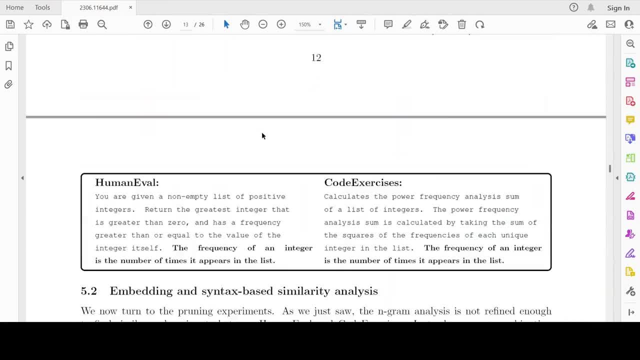 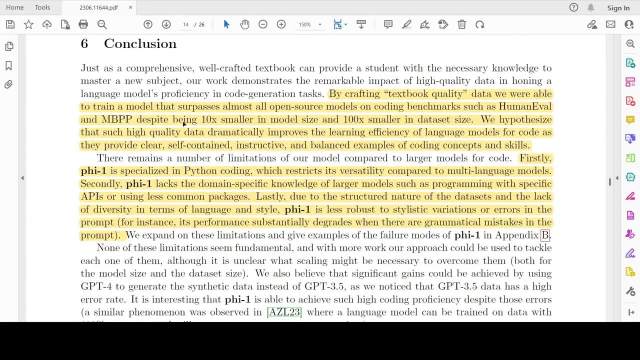 So if I go to the conclusions over here, what this paper says is that, you know, by crafting textbook quality data, we are able to train a model that surpasses almost all open source model on coding benchmarks, despite being 10x smaller in model size and 100x smaller in data set size. 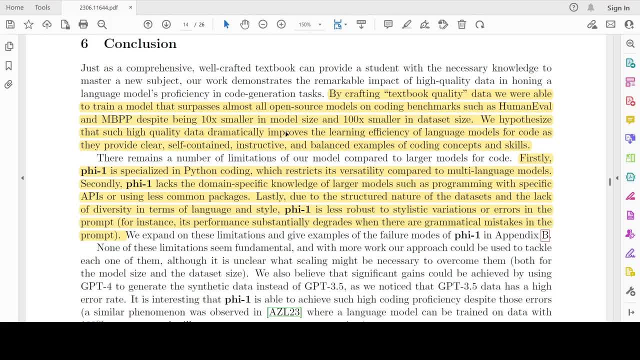 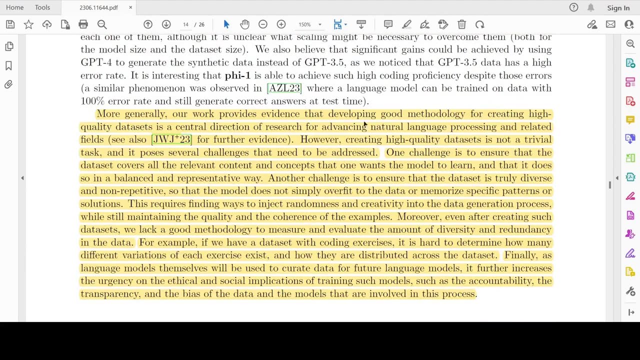 so they hypothesize that such high quality data dramatically improves the learning efficiency of language models for code as they provide clear self-contained instructive and balanced examples of coding concepts and skills okay but there are some limitations over here so this is like if you have high quality data even smaller models can give you very good results that is a kind of conclusion and insight okay sick but they are saying that there are some limitations it is only specialized in python coding okay which restricts its versatility compared to multi language models it also lacks domain specific knowledge of larger models such as programming specify apis or using less common packages okay due to the structured nature of the data set and lack of diversity in terms of language and style it is less robust to stylistic variation or error is in the prompt okay stylistic variations or error it degrades basically performance substantially degrades when the grammatical mistakes in the prompt so this is uh you know 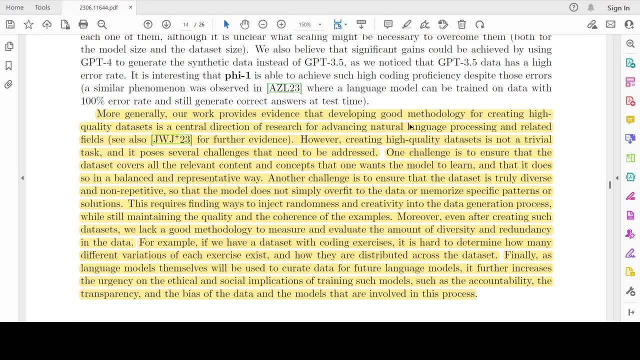 this is a very good insight that how can you create high quality data set okay it is not it is not a trivial task there are several challenges which needs to be addressed one is like you need to ensure that the data set covers all the relevant content and concepts that one wants to the model to learn